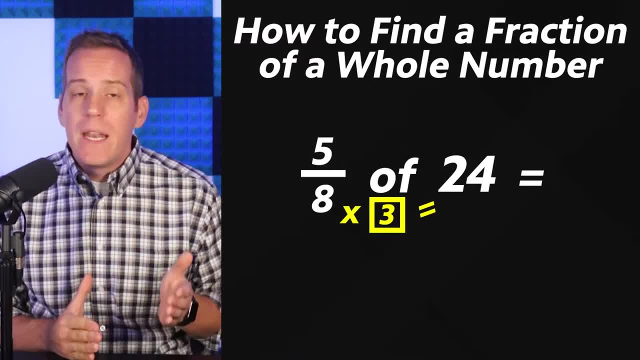 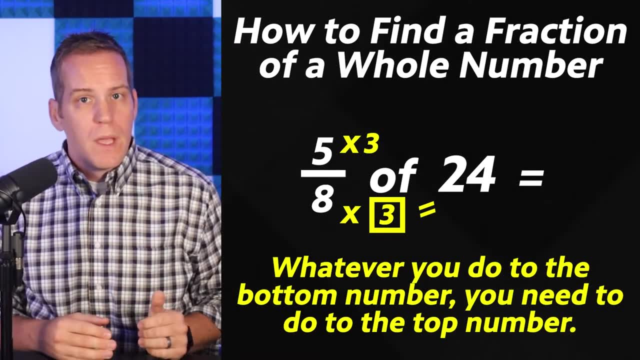 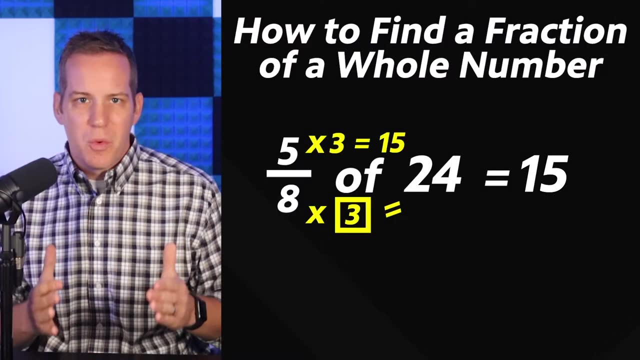 Okay, now, if I do times three on the bottom, I need to do times three on the top. Okay, whatever I do to the bottom number, I need to do to the top number. So five times three is 15.. And guess what? That's the answer: Five eighths of 24 is 15.. Now how the heck did that work? 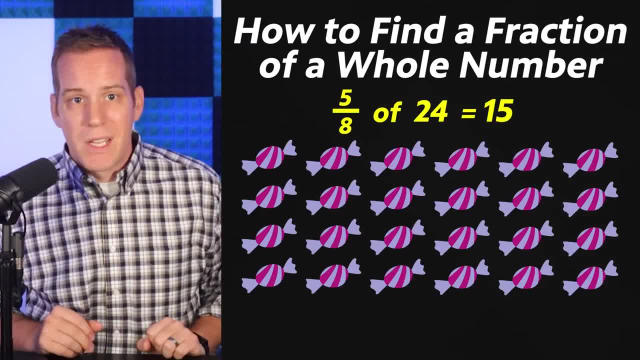 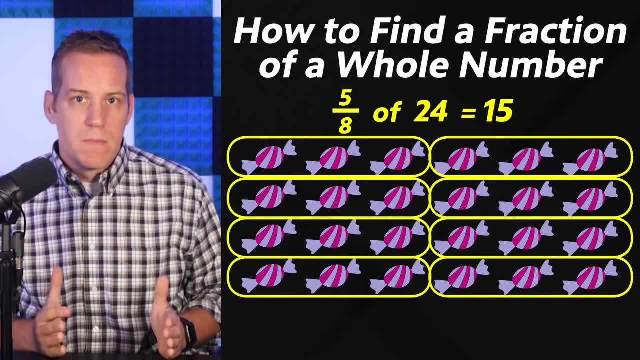 Well, let's look at this model. All right, let's look at those 24 candies again. To find five eighths would mean I need to first split the 24 candies into eight equal groups. Each of these groups is one eighth of 24.. 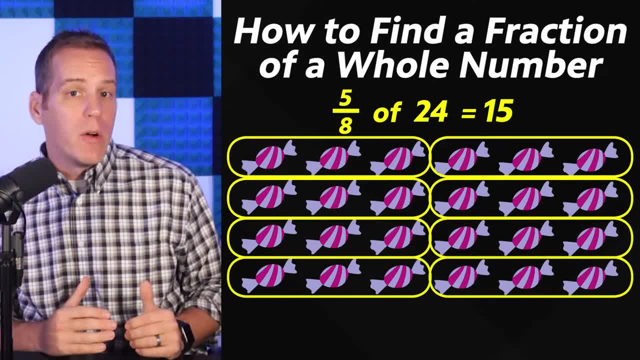 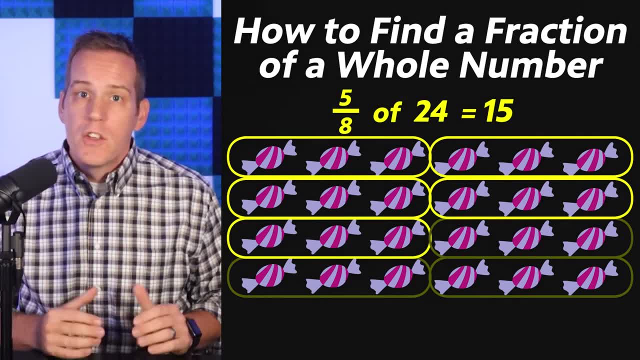 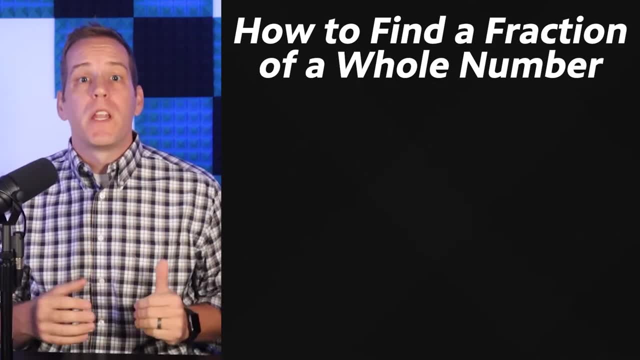 So to find five eighths, I would need to know how many are in five groups, And that's easy right. Five of these groups would make 15.. So what I showed you earlier is kind of the shortcut for solving this type of problem. Now let's switch up the numbers and do a. 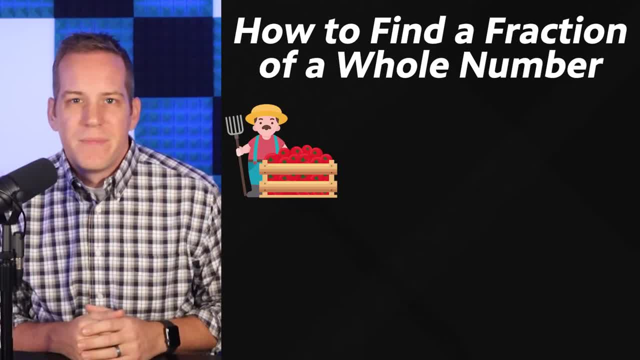 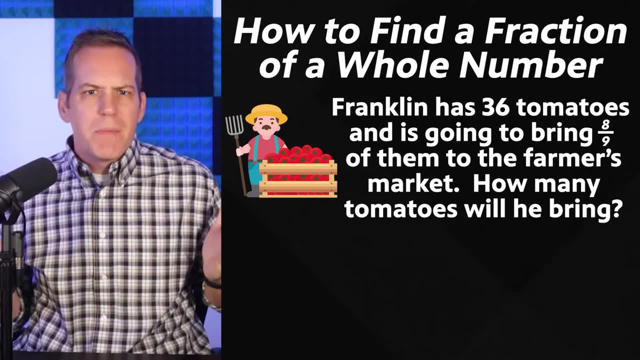 different problem. Okay, let's meet Franklin. Franklin has 36 tomatoes and is going to bring eight ninths of them to the farmer's market. So how many tomatoes would he bring? The math problem here is: what is eight ninths of 36.. 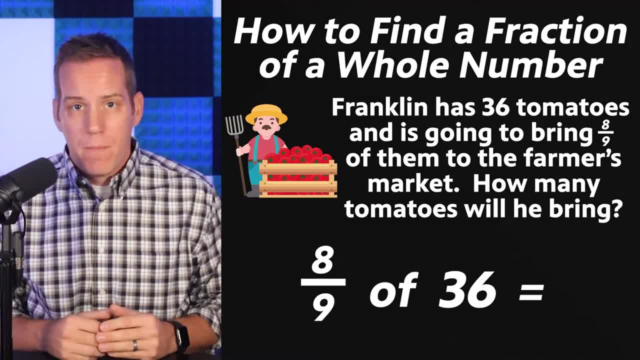 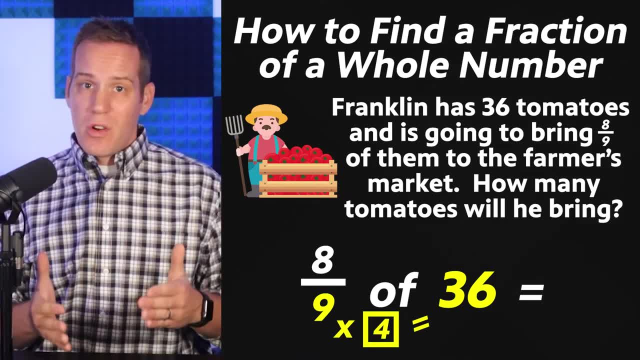 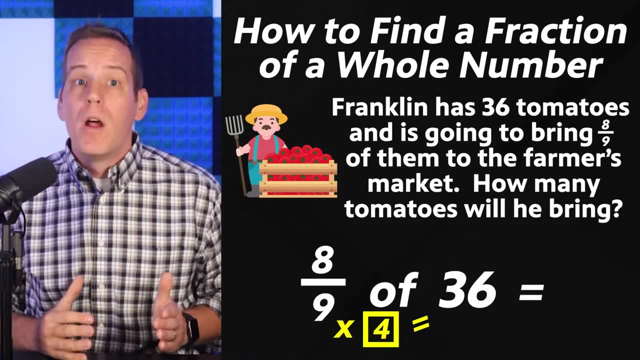 So start by looking at the denominator and the whole number. Can nine go into 36? perfectly? You bet it can. Nine times four equals 36.. So I'm going to put a times four next to the nine And just like before, whatever I do to the bottom number, I'll do to the top number. 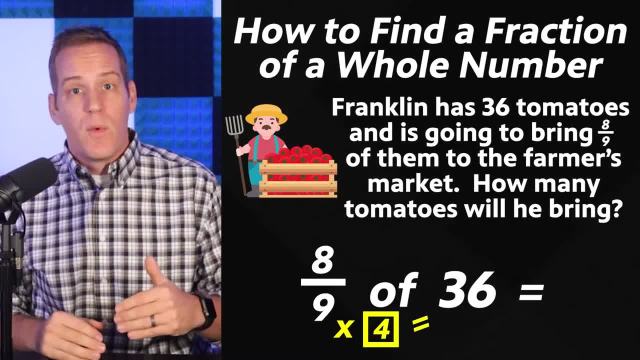 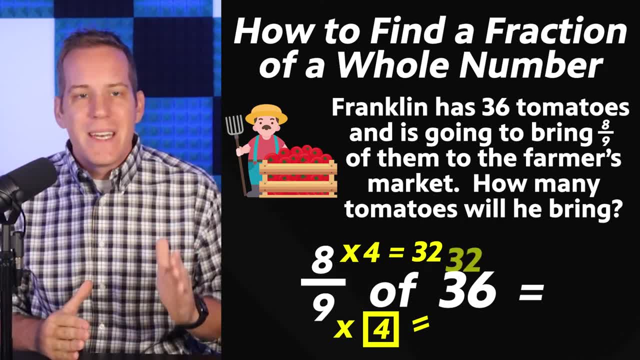 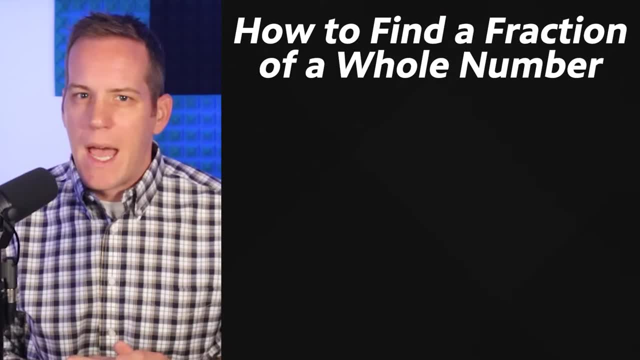 So if I do times four on the bottom, I'm going to do times four on the top. So what is eight times four 32.. And that's the answer. Eight ninths of 36 equals 32.. But now let's crank the difficulty level just a tad. 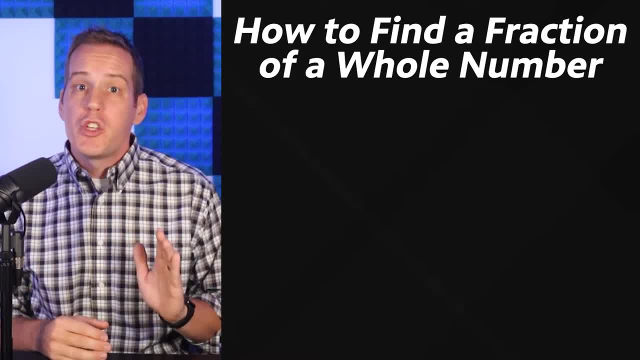 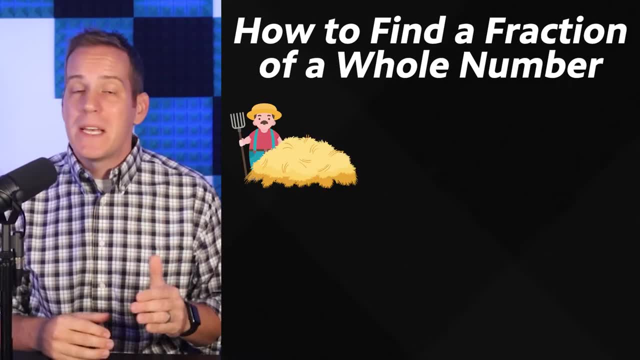 Remember how I said there'd be a harder way to do this too. Well, let me show you why you might have to use that harder strategy. Let's go back to our old pal Franklin. This time he has to feed some horses. He has 13 bales of hay. 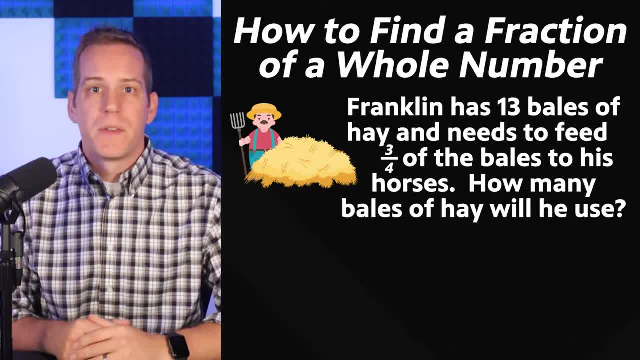 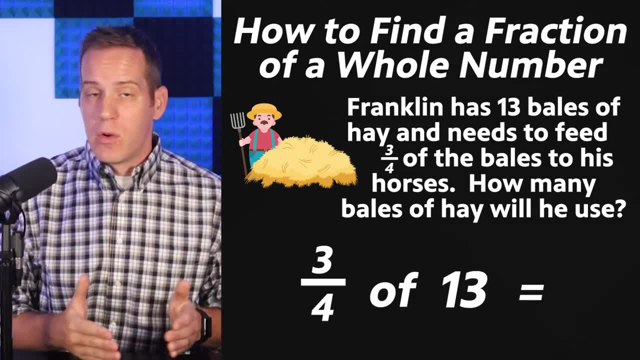 and he needs to feed three fourths of those bales to the horses. How many bales of hay is that? The math problem here is this: What is three fourths of 13?? If we try our other strategy, we'd have some problems. 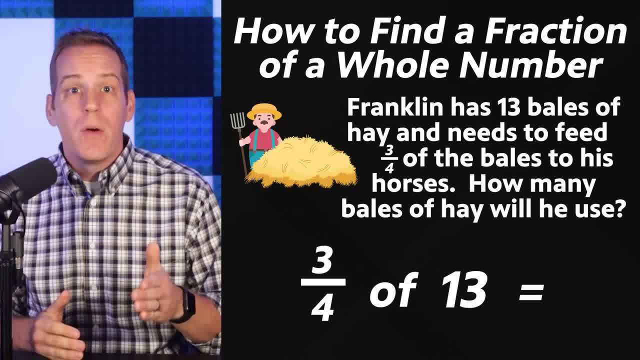 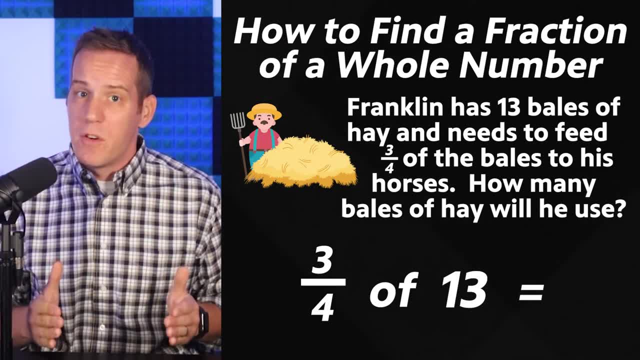 Can you see why? It's because four can't go into 13 perfectly. If I count by fours, I won't land on 13. So I can't do that first strategy. When this happens, don't sweat it. All you have to do is turn this problem. 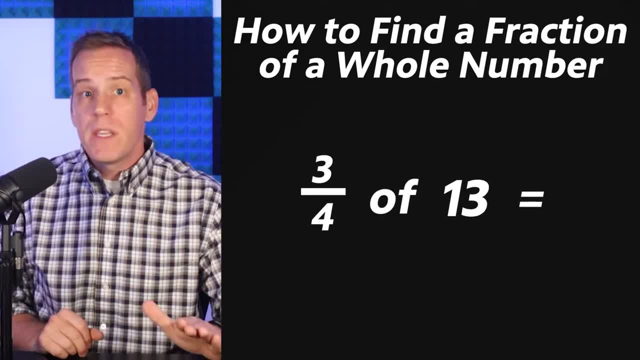 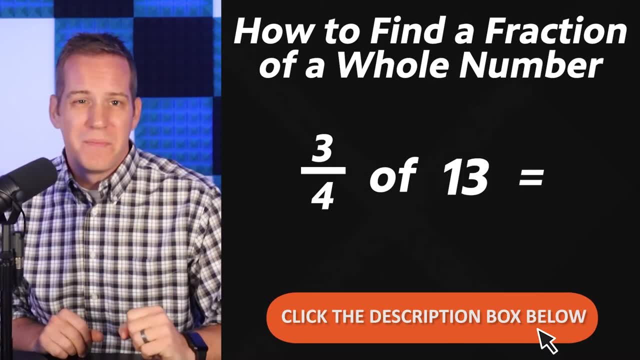 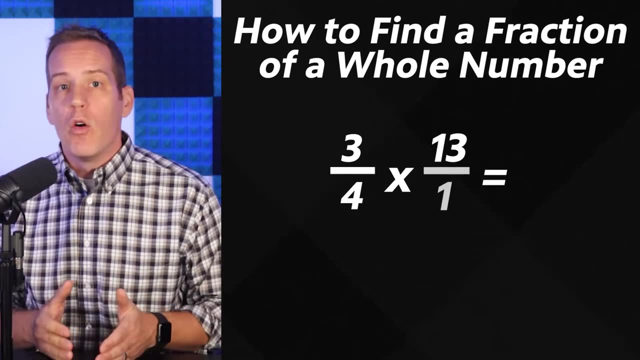 into a fraction multiplication problem. Now we've covered this in a previous lesson, So if you need more practice with multiplying fractions by whole numbers, click the description box or click the link up here. Three fourths times 13 is going to become three fourths times 13 over one. 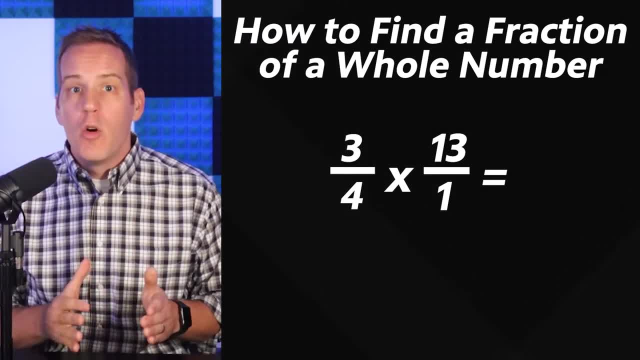 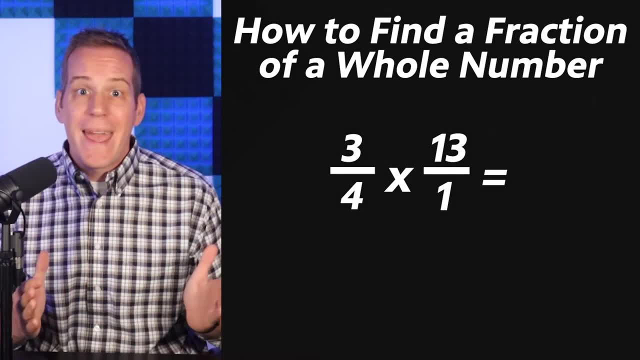 Because, as you may remember, when you multiply by a whole number, you always write that whole number as a fraction over one. Now we check for cross simplifying, but we can't in this problem, So we're gonna go right into multiplying straight across. 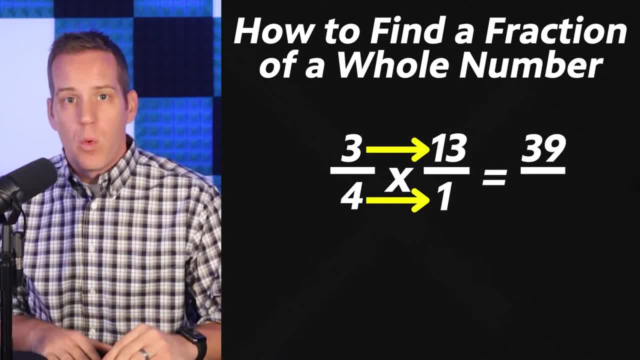 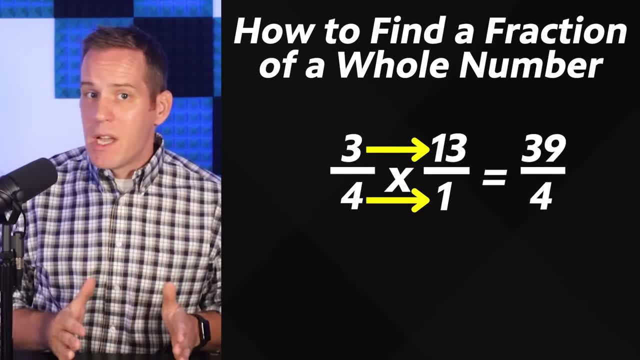 Three times 13 is 39, and four times one is four, So I've got 39 over four. Now I need to turn this back into a mixed number, since 39 over four is improper, And that's just division. Four goes into 39 nine times. 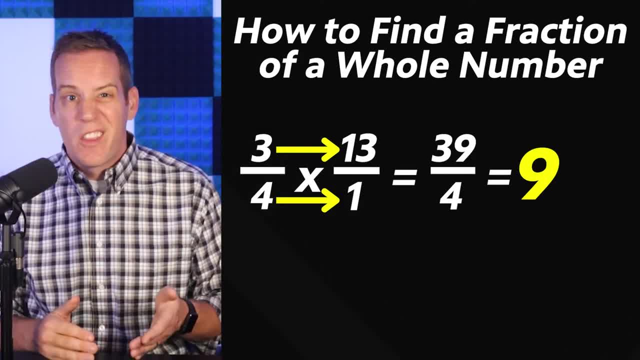 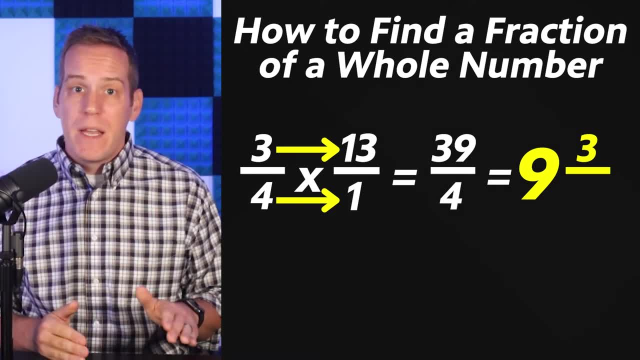 So that's our whole number. Now, four times nine is 36. And it'd take three more to count up to 39. So three becomes our numerator. The denominator stays the same. So we have our final answer, which is nine and three fourths. 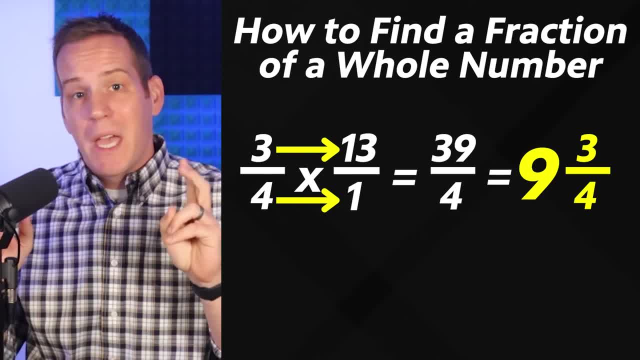 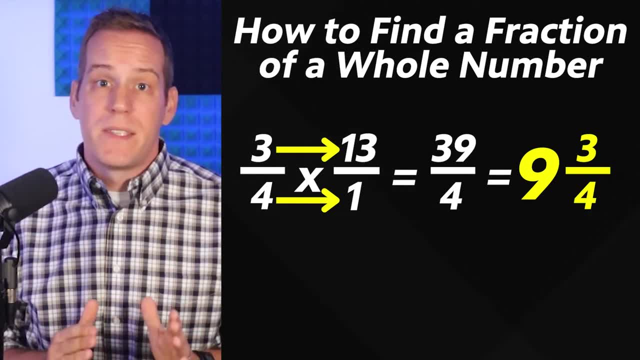 By the way, for what it's worth. you can use the turn it into a multiplication problem for any fraction of a whole number problems, even the easier ones we did earlier. However, as a teacher, my advice is this: If you have an easier method, 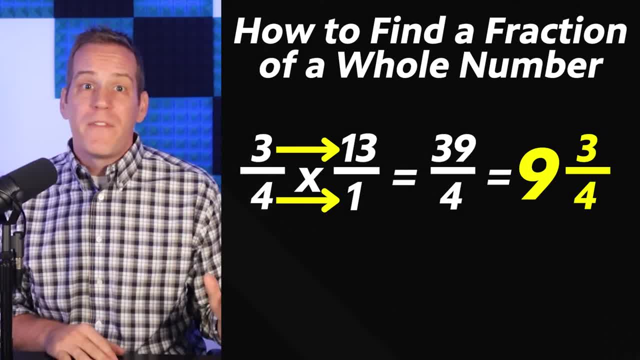 that can get you the right answer. do it. Math is all about finding the simplest way to do it. Math is all about finding the simplest way to do it. Math is all about finding the simplest way to calculate the right answer. So if you have a math shortcut, use it. 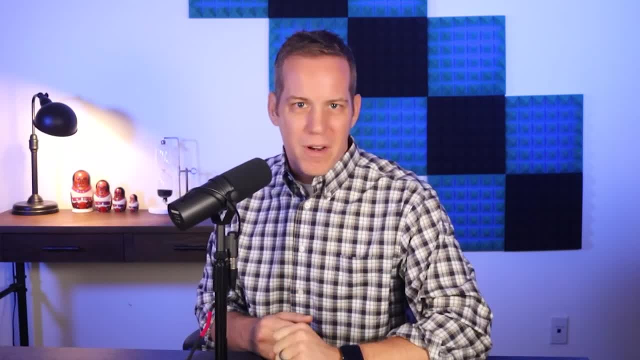 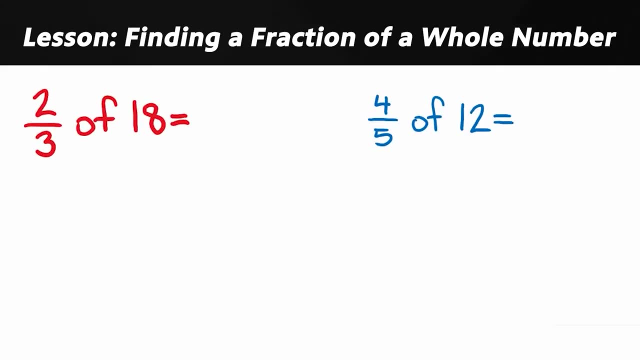 Okay, practice time. Grab your paper and pencil and let's go to the whiteboard. I've got two different problems for you to look at. They're both asking to find a fraction of a whole number. Can you see which one we use the easy strategy with?